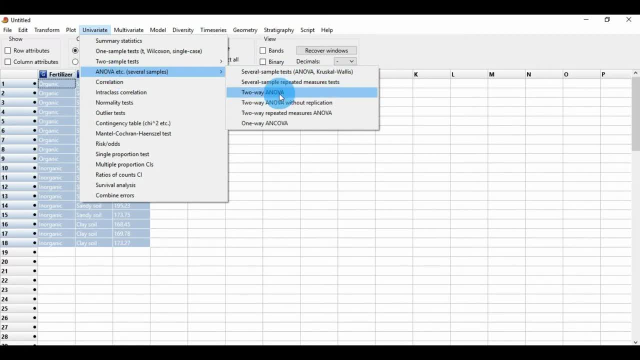 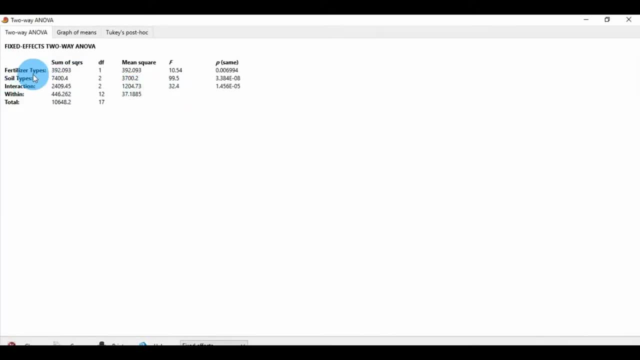 markets- anava. click the two anava Now open the new window. this is for the two anava table. Custom. the fertilizer type: The sum of square value: 392.093,. the difference of freedom df for one, the mean of square 392.093.. The F value for the 10point 54. the p value: the. 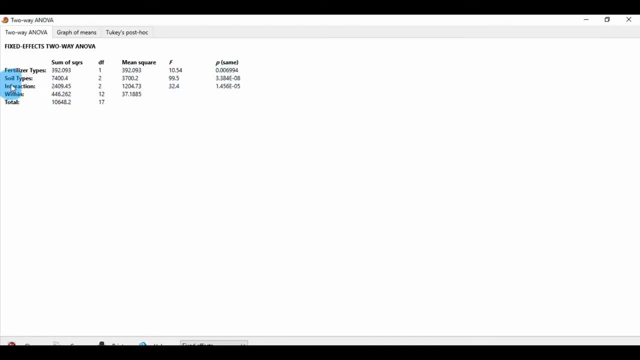 less than 0.05. so it's a significant value, and another one, the soil type. the soil type: sum of square value 7400 and the difference of freedom to the mean square 3700. the f value 99.5. the p value non-significant because the higher than the 0.05, and the interaction for the 2409. 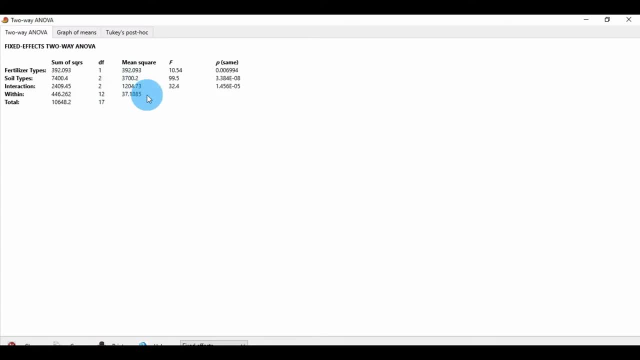 and the difference of rate to the mean of square 1204, the f value: 32.4. the p value, also non-significant. the within the value sum of square 446. and the difference of freedom to the mean square 37.1885. the total of sum of square 10648.2. the total difference of freedom. 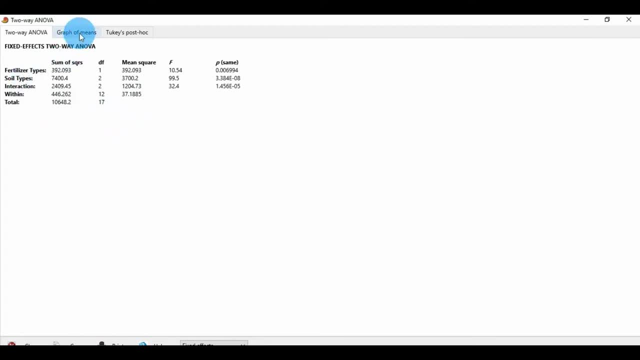 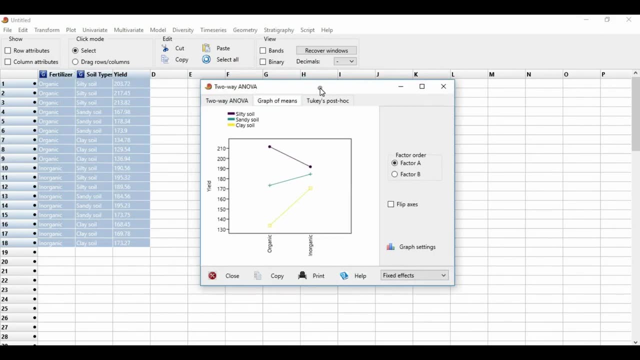 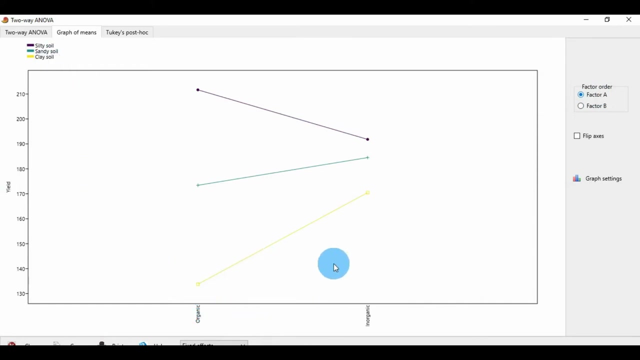 the 17. the another one menu for the graph, the. this is two-way graph. the first one, the factor a and the factor v, because the factor a for the fertilizer type, organic and inorganic. the second one factor for the soil type, three type of soil type. first we know the fertilizer a, the organic fertilizer, low production by the sandy soil and 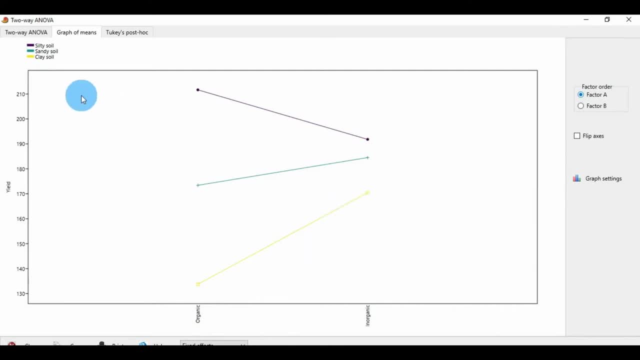 the high production for the inorganic soil and also clay soils, the low production for the organic and the high production for the inorganic sample and the factor b. this is a factor b, the production value, the silly soil, sandy soil and clay soils. now on the another one for the 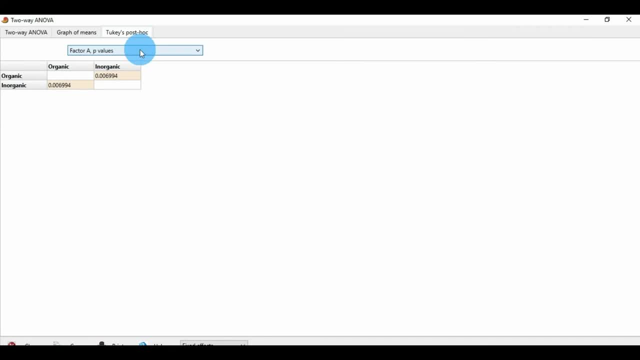 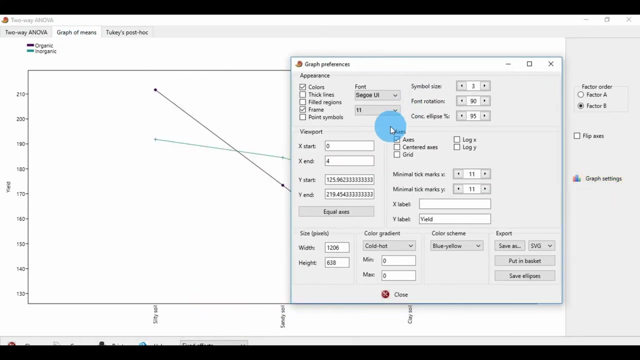 post-work test. the four blocks are the factor a- p value and the factor a q values and factor b- p values and the factor b q values and the interaction values. now the export for the two and our graph, the to the two anava graph menu and go to the graph setting menu. click the button, the open the new.